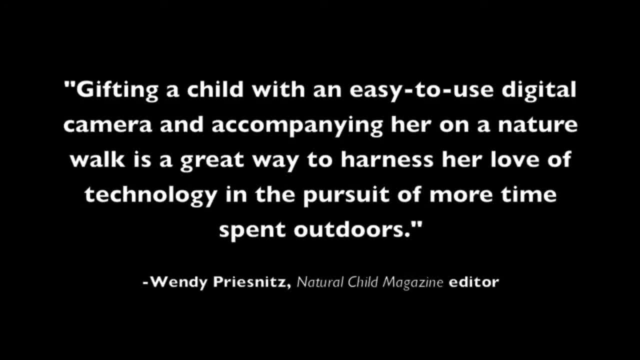 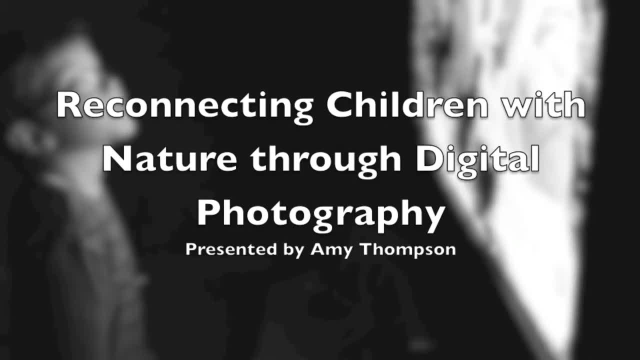 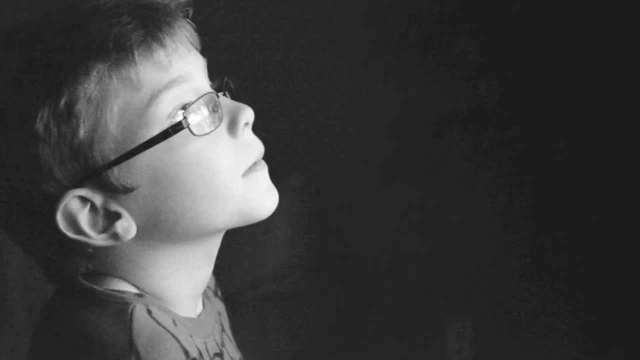 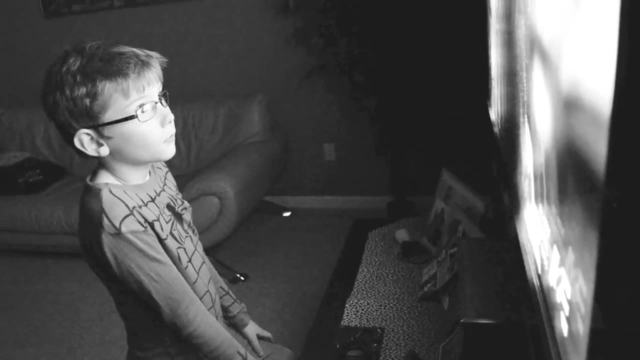 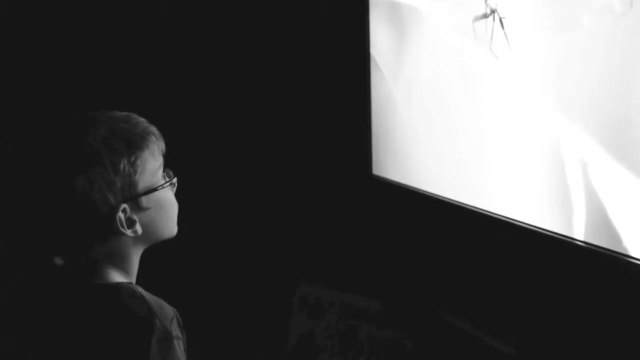 Take a few seconds and look at this face. Does the blank stare look familiar? Are we turning our children into zombies by putting them in front of high definition screens for hours on end? Isn't there something less mind-numbing that they could be doing? I mean? 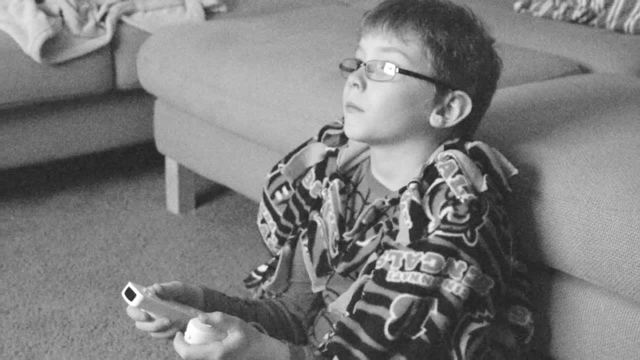 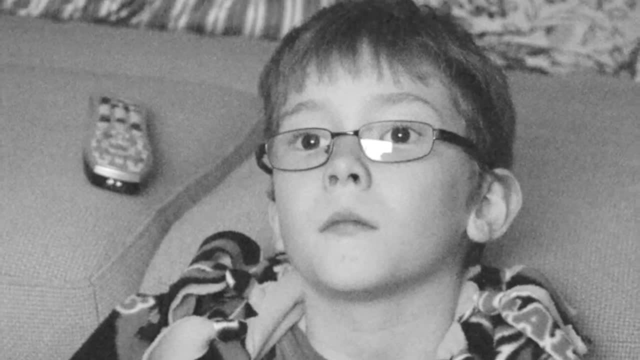 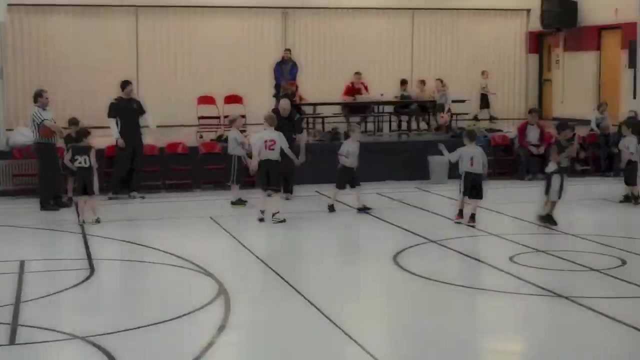 really look at this face. Doesn't he deserve something more? As parents today, we struggle in many ways to do what's best for our children. Today's fast-paced technological world has ever-increasing options for indoor recreation. Because of this, kids are. 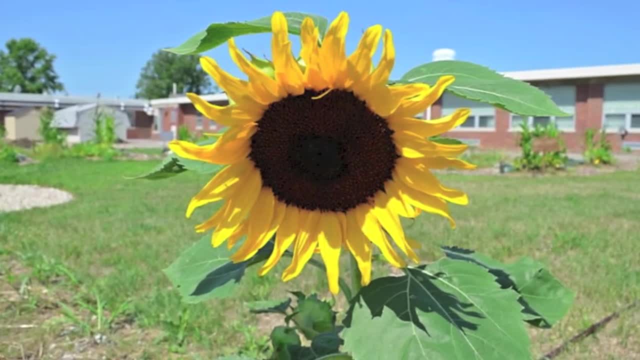 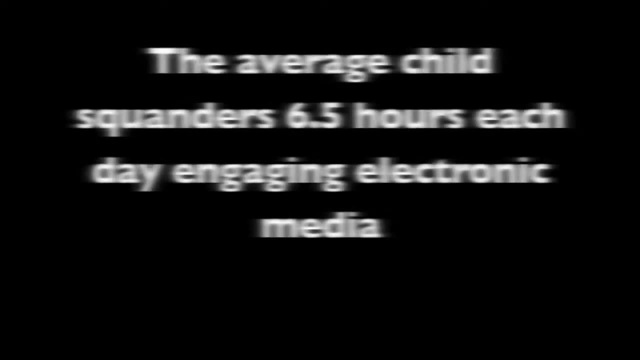 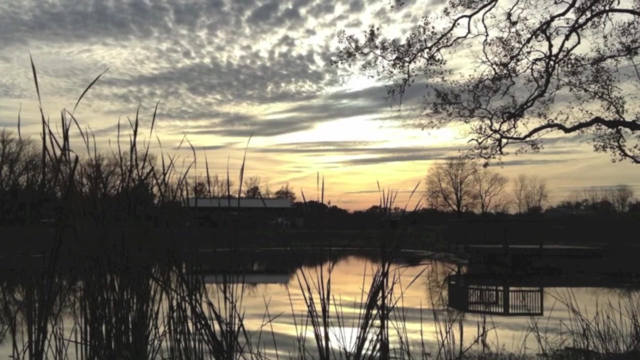 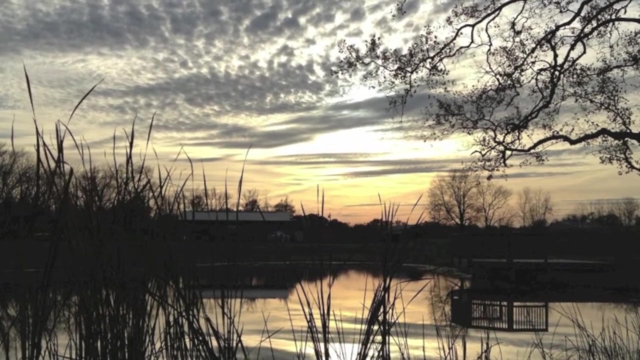 rapidly losing their ancestral desire to get outdoors and play. I bet that if you're anything like me as a child, your parents probably sent you outdoors early in the morning and expected you to spend the majority of your day outside riding bikes and climbing trees. But something's changed since we were children. 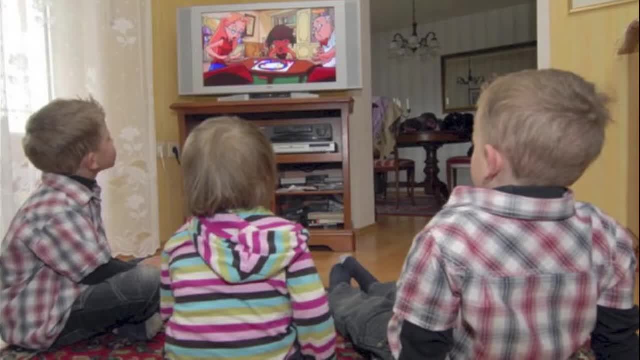 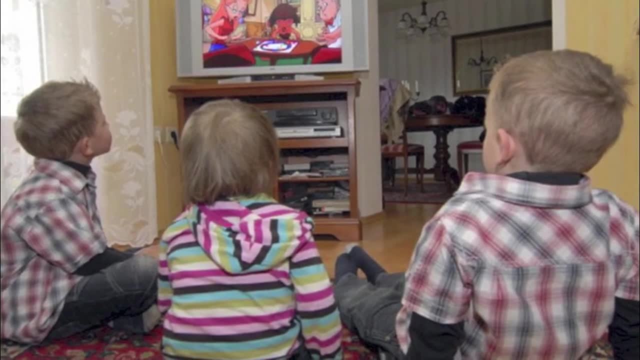 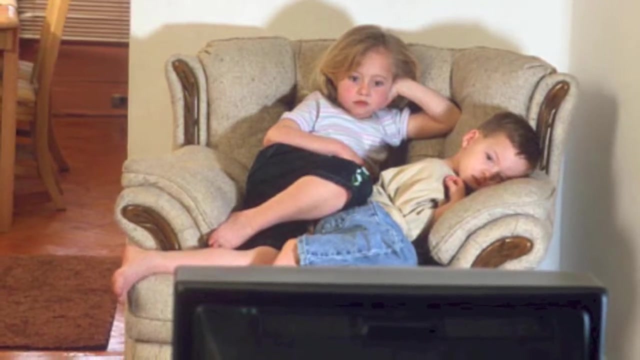 It's become easier and perhaps even safer for parents to simply turn on a TV and put in a DVD or hook up a video game than it is to send their children outdoors. What my generation needs to realize is that what may be easiest may not be the best thing for our children. In fact, some of 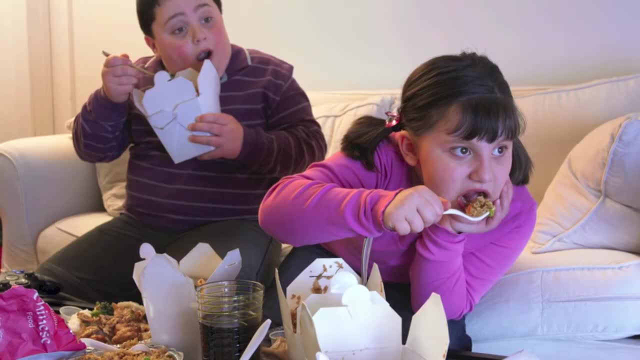 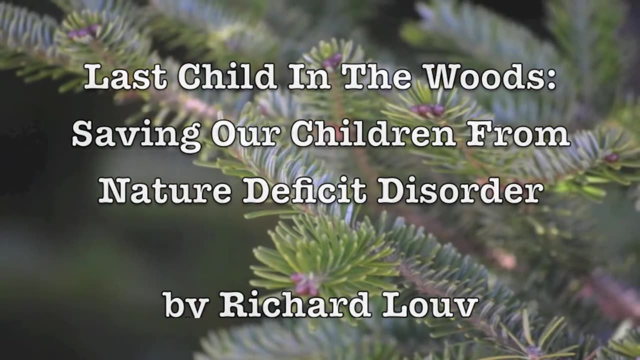 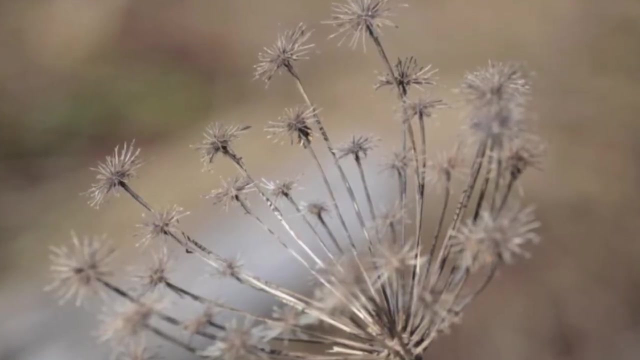 these choices may be making your children sick, lazy and unappreciative of all that nature has to offer. Richard Louv really is the book that all parents should read. In this book, Richard describes our children's lack of connection with the natural world, What he describes as nature deficit disorder. 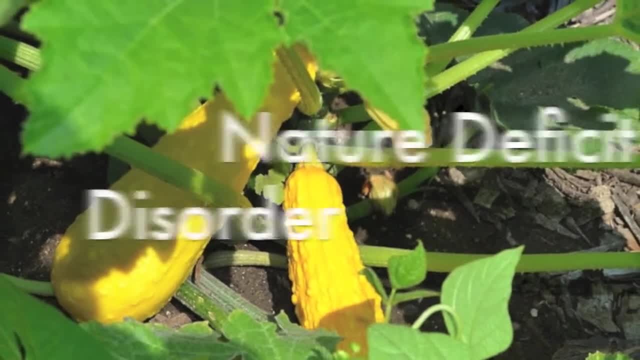 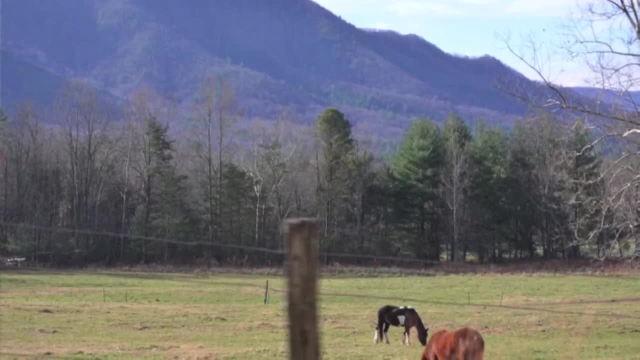 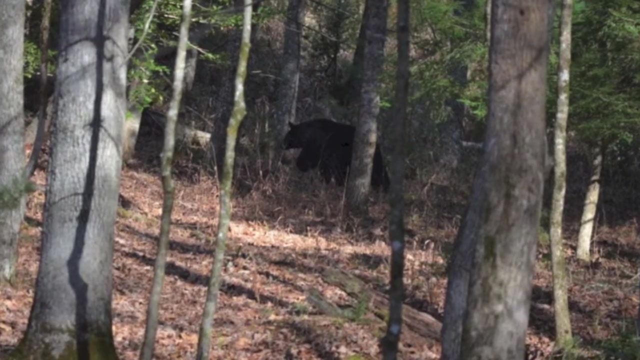 is not a medical condition that a pediatrician can diagnose, but it does tend to act like a disease, attacking children and families and even entire communities. Sadly, playtime is decreasing and screen time is increasing for our children. So too is the likelihood that our children will be overwhelmed by the pandemic. So let's take a look at some of 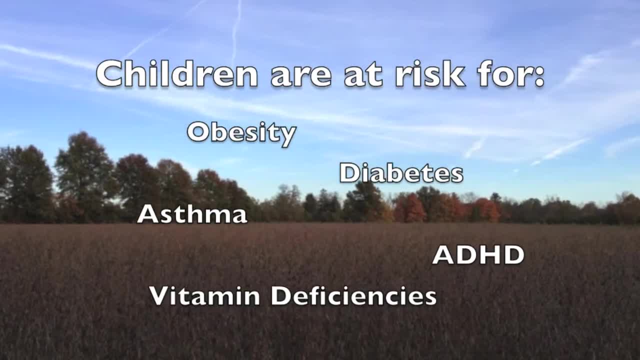 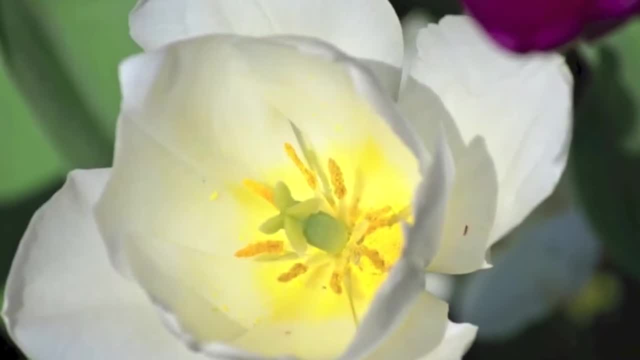 these leading factors that may be making our children sick. Many of these factors may be associated with weight or suffer from other serious health problems, including type 2 diabetes, asthma, ADHD and even vitamin deficiencies. Is it actually possible that today's digital natives, who've grown up with technology, may be at risk of living shorter? 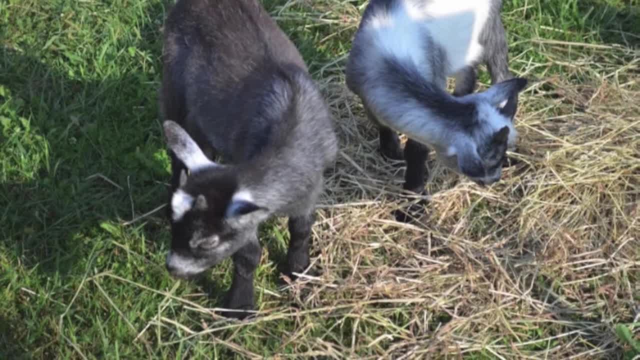 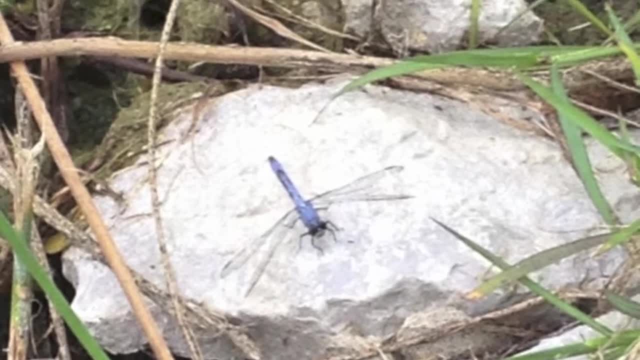 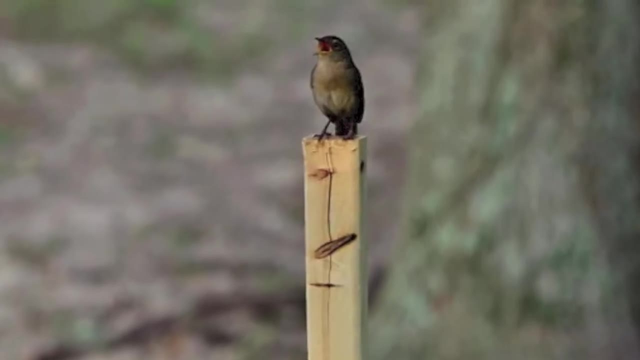 less healthy lives than us, their parents? Now, that's a scary thought, But we have something else to worry about too. Our children's growing lack of knowledge about nature and wildlife could have real and serious consequences- consequences for our planet, For one thing. how will children develop a sense of responsibility? 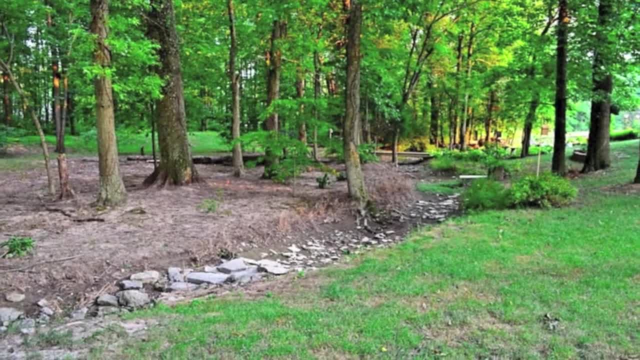 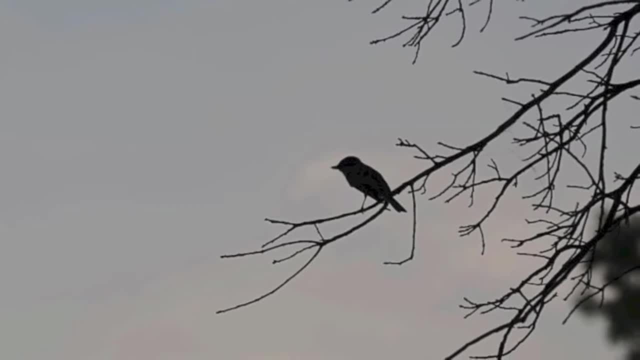 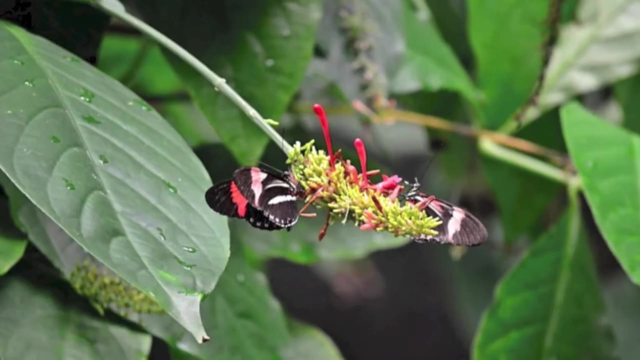 for protecting the diversity of life on earth if they know little to nothing about it? How will we create the next generation of environmental stewards if our kids aren't taught to value nature? Clearly, we all want our children to be safe, but we cannot expect them to live inside a bubble. 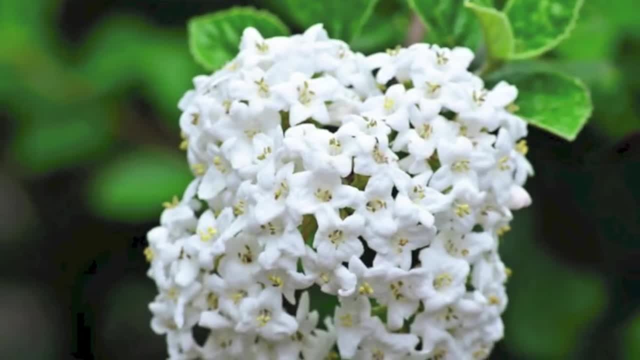 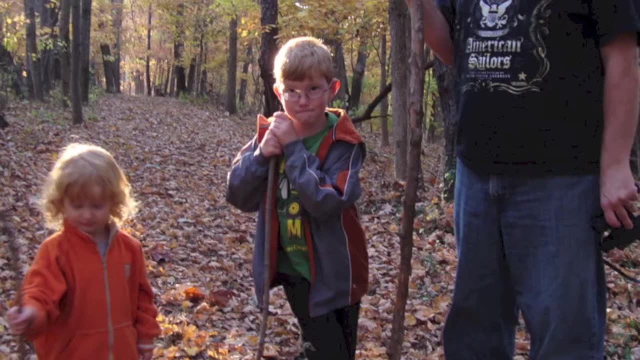 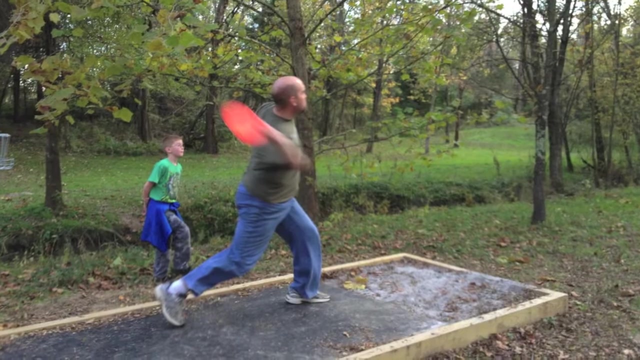 When kids go outside, there will always be the potential for insect bites, sunburns and broken bones, but we cannot let our fears overwhelm us. So, parents, let's get up off the sofa and lead by example, encouraging our kids to go outside by joining. 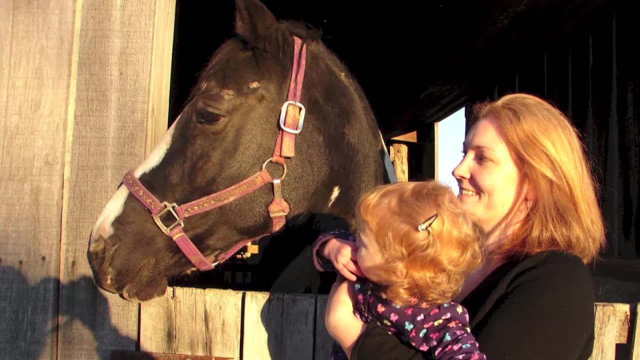 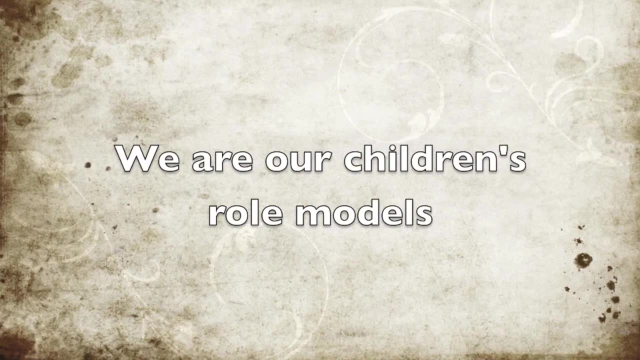 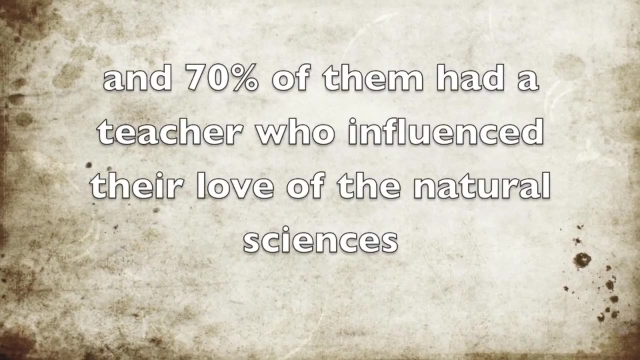 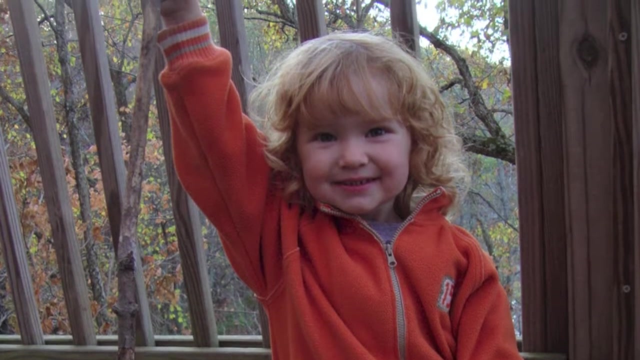 them. If we can commit to this, we'll make family outdoor activity more likely. Nature was our first classroom and it's always been the best classroom. It's been said that perhaps the most effective prescription for what ails us is a heavy dose of nature. 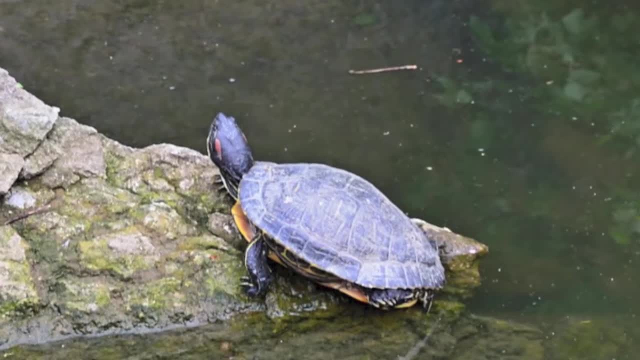 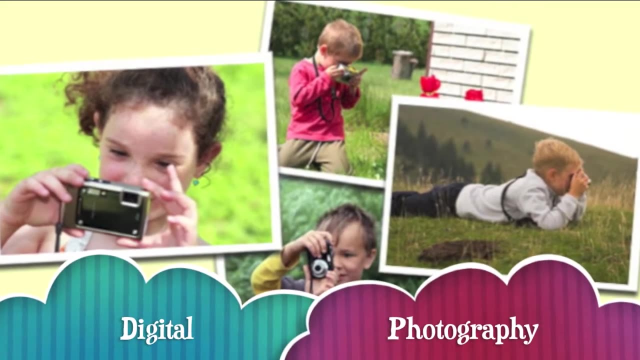 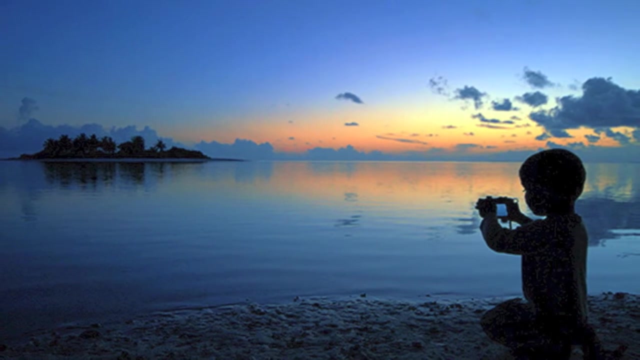 and I truly believe that. So, parents, if you're ready, let me show you one way to reconnect your children with nature. That option is through the use of digital photography. Wait a minute. What's that you said? Didn't you just talk about how bad technology was for kids? 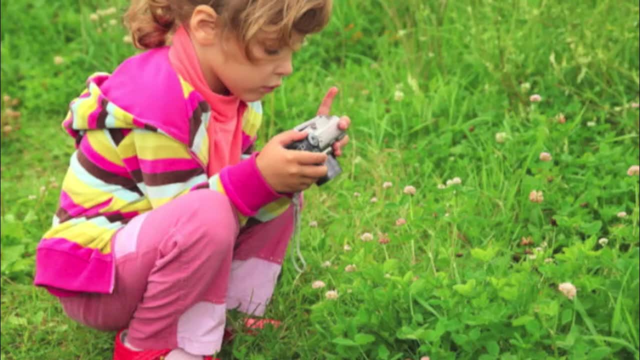 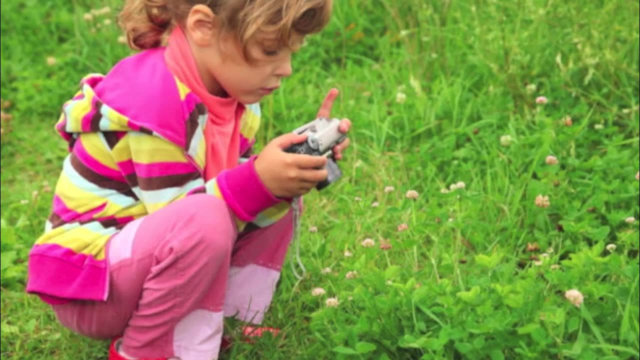 Is it possible that something as simple as giving a kid a digital camera and sending them out into nature may actually lead them down a path towards reconnection with nature? Well, yeah, actually Giving kids access to digital cameras puts them in the driver's seat and allows them to control. 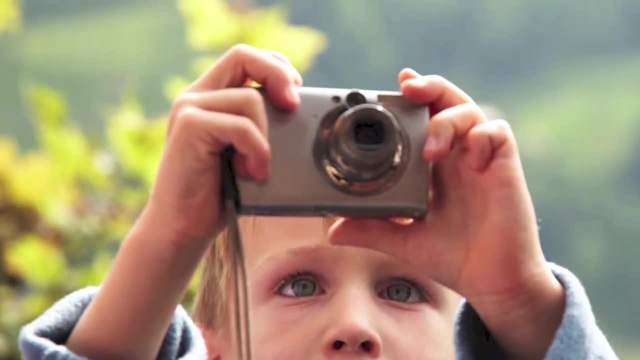 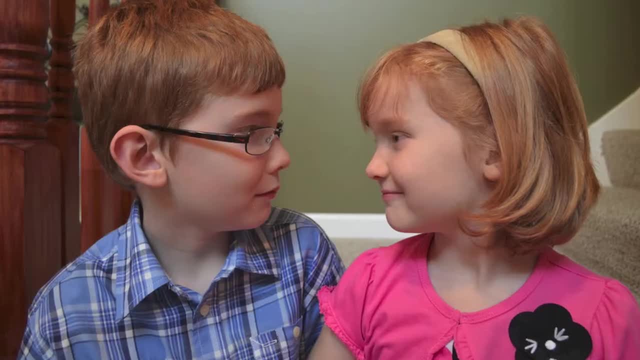 example to a child. I gave my example to a child. I gave my example to a child. I gave my example to a child. Hi, Glenn, how are you? I'm spending my own two children- digital cameras and set them free to explore. 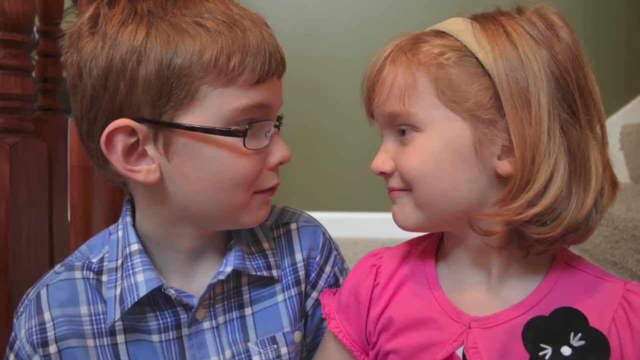 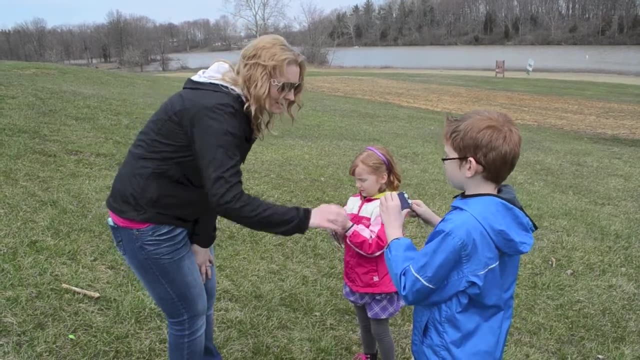 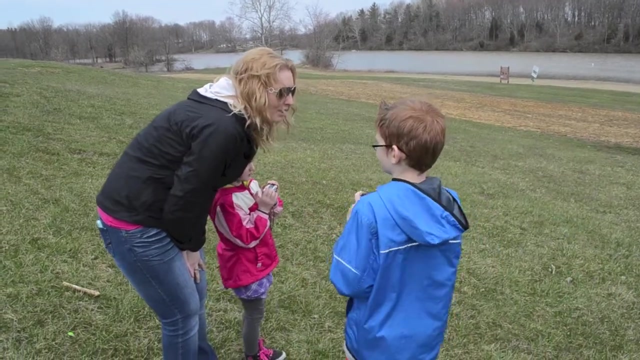 nature, documenting whatever they found interesting. The result is simply amazing. Alright, here you go, Here's your cameras, And what I want you guys to do is turn them on. You got it on, Okay, push the power button And I want you guys to go out. and here at, 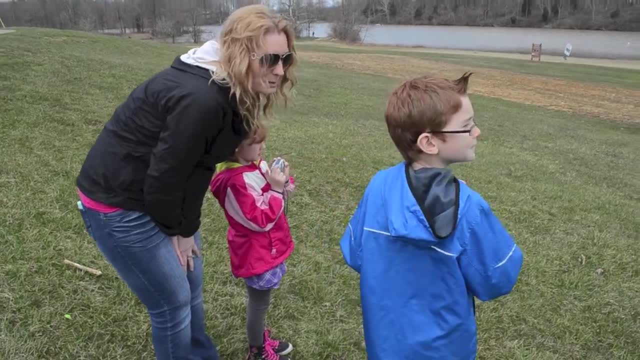 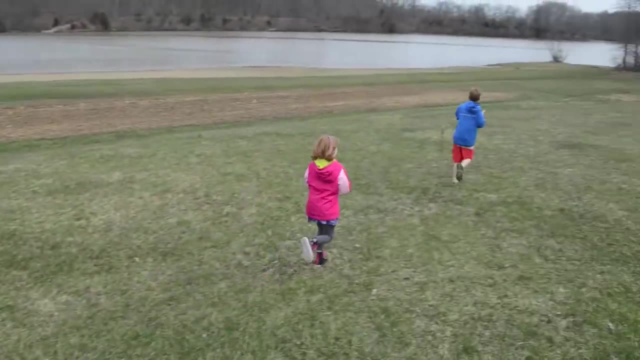 the park to take pictures of whatever is interesting to you, Whatever in nature makes you happy and be excited. go take a picture of it. okay, Alright, have fun. We're the children of tomorrow. dream away in the wind of change. 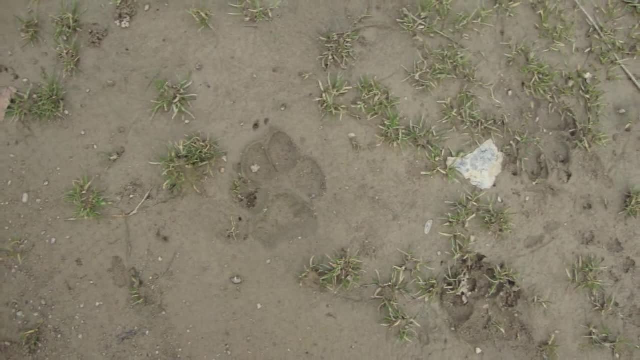 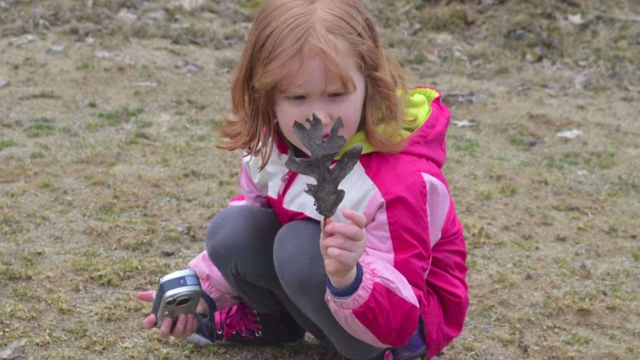 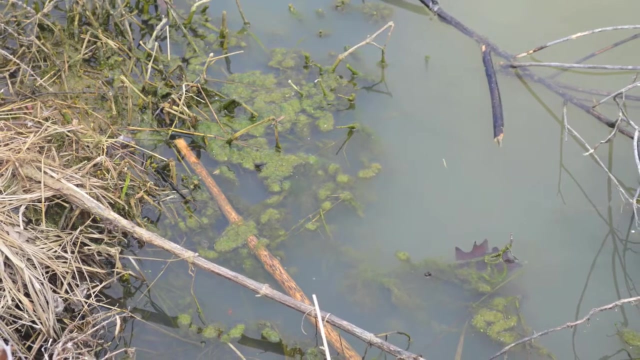 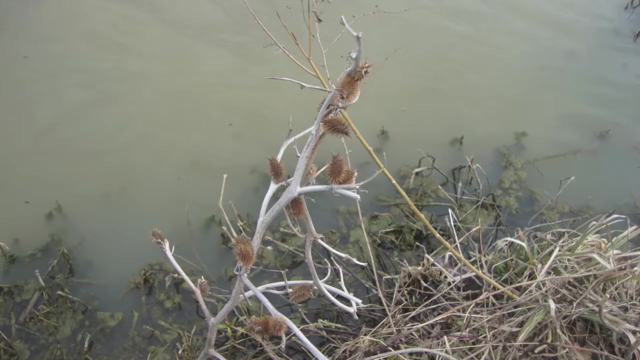 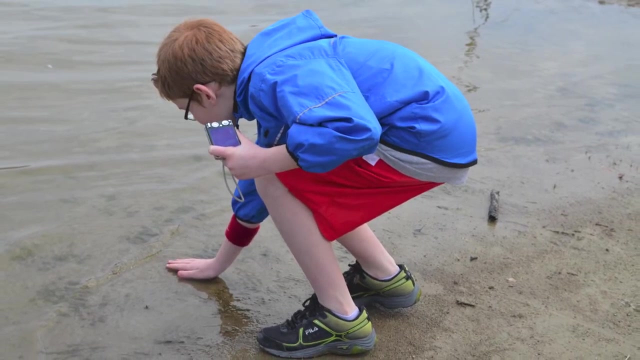 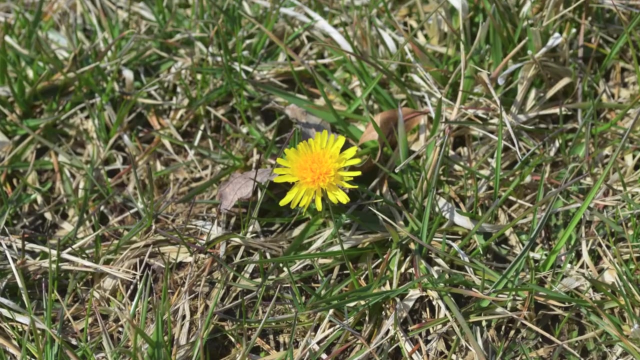 Did you think that your feet had been bound by what gravity brings to the ground? Did you feel you were tricked by the future you picked? Well, come on down. All these rules don't apply when you're high in the sky, So come on down. 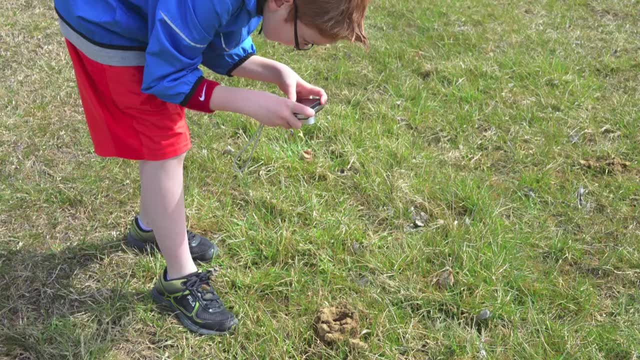 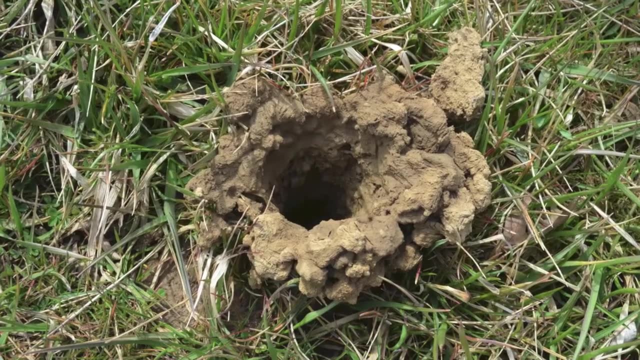 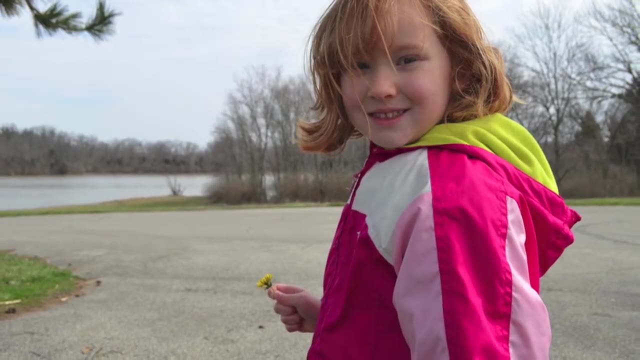 Come on down. We're coming down to the ground. There's no better place to go. We've got snow upon the mountains. We've got rivers down below. We're coming down to the ground. It's been suggested that methods that integrate both technology and nature. 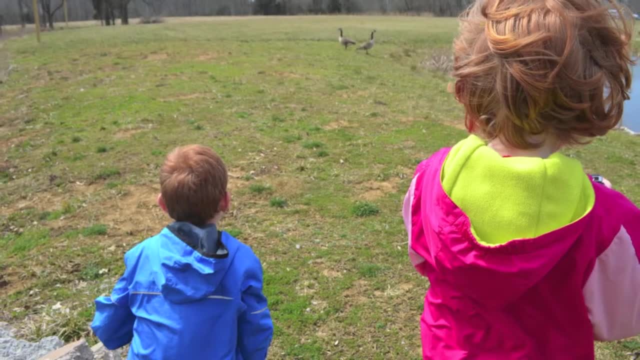 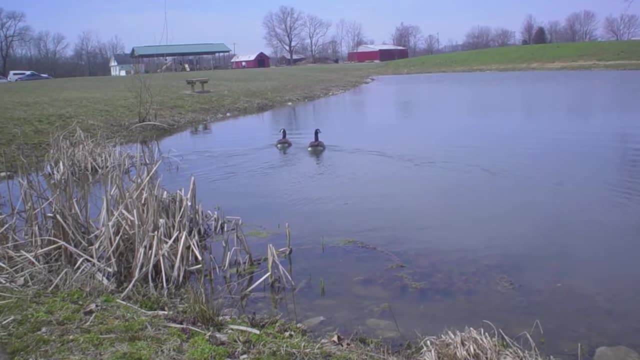 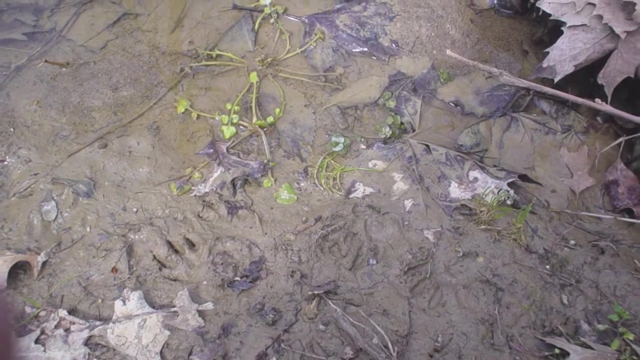 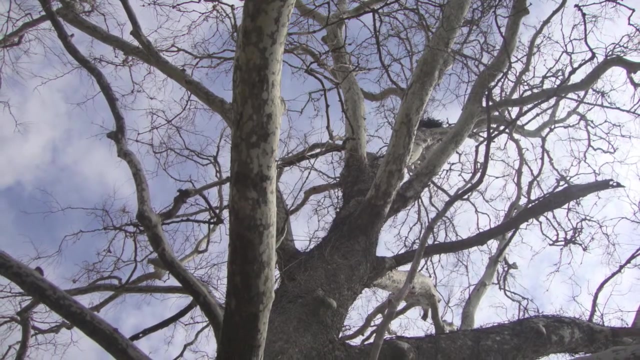 rather than ignoring technology completely, will be most effective for reaching today's youth. Did you think you'd escaped from routine By changing the script and the script, By changing the scene. Despite all you've made of it, you're always afraid of a change. 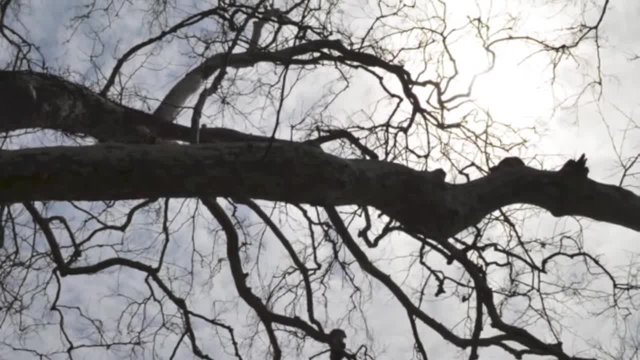 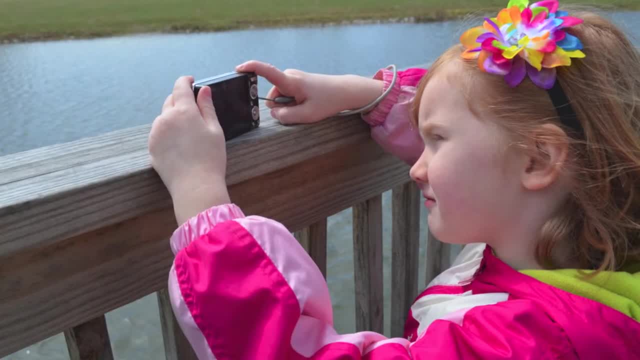 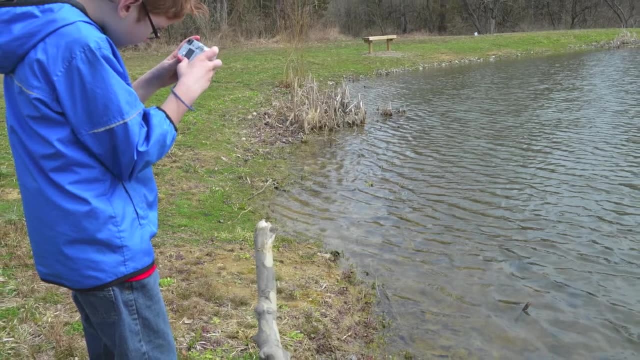 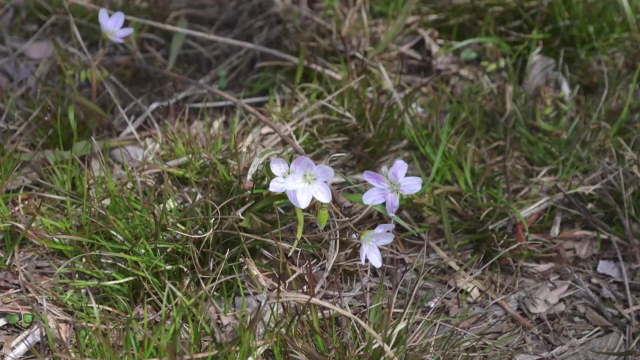 You've got a lot on your chest. Well, you can come as my guest. So come on down. Come on down. We're coming down to the ground. There's no better place to go. We've got snow upon the mountains. 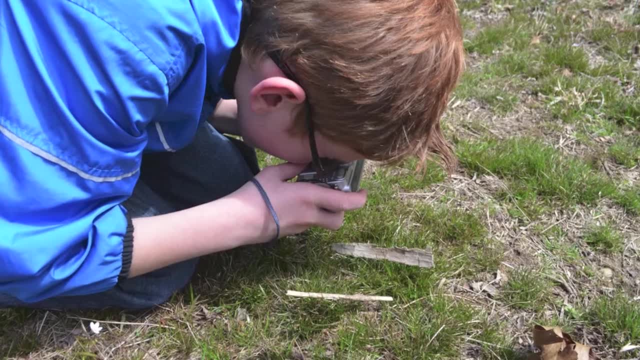 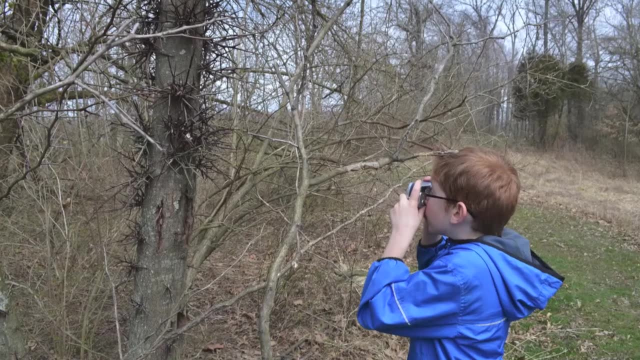 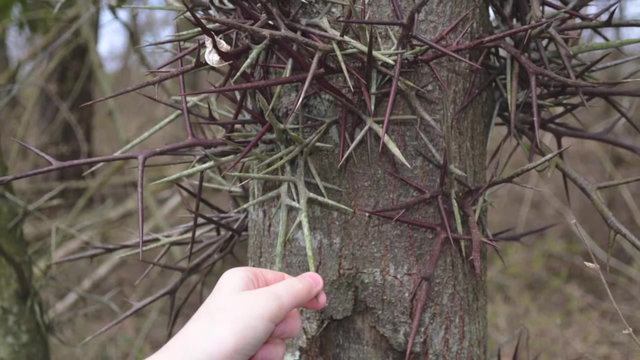 We've got rivers down below. We're coming down to the ground, We hear the birds singing in the trees And the land. we're feeling after We send the seeds out in the breeze, Like the fish in the ocean. Like the fish in the ocean. 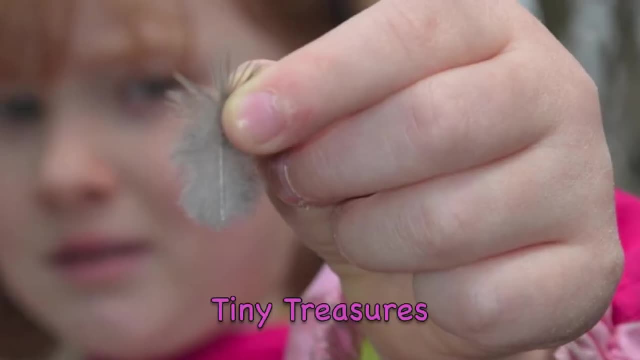 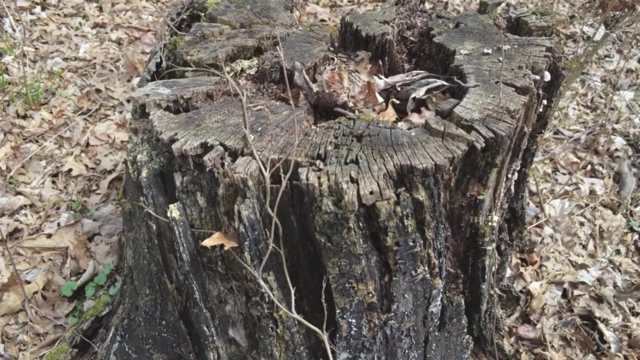 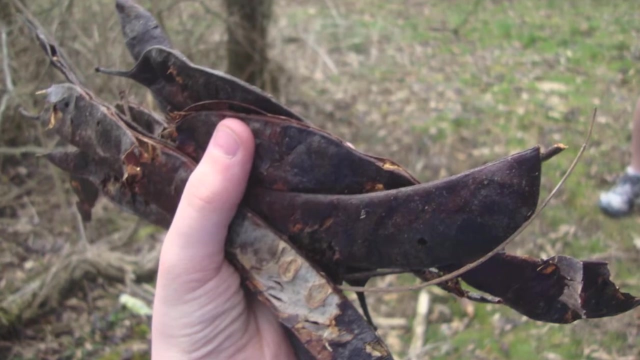 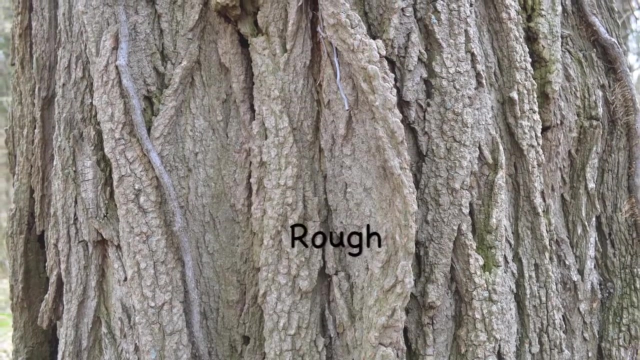 We felt at home in the sea. We learned to live off the good land. We learned to climb up a tree, Then we got up on two legs, But we wanted to fly. And when we messed up our homeland, We set sail for the sky. 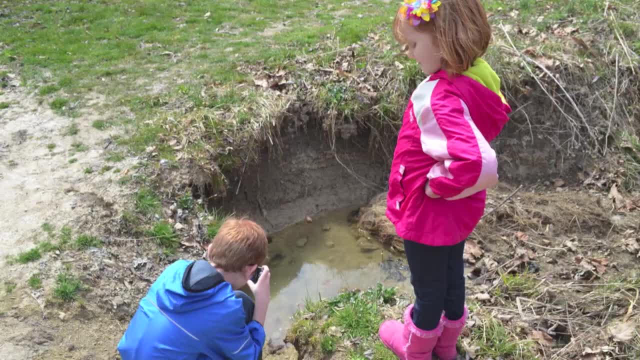 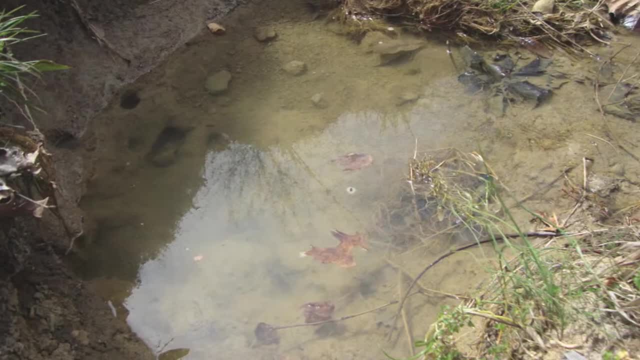 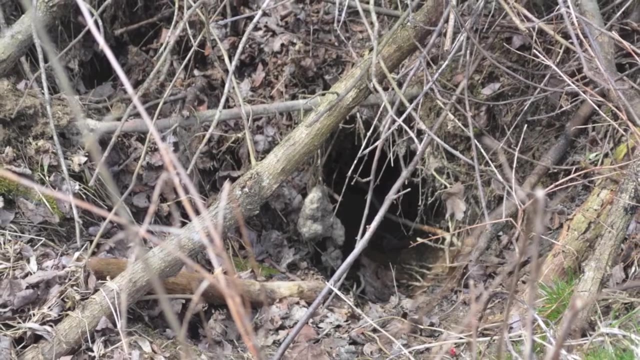 We're coming down to the ground. There's no better place to go. We've got snow upon the mountains, We've got rivers down below. We're coming down to the ground. We hear the birds singing in the trees And the land. we're feeling after. 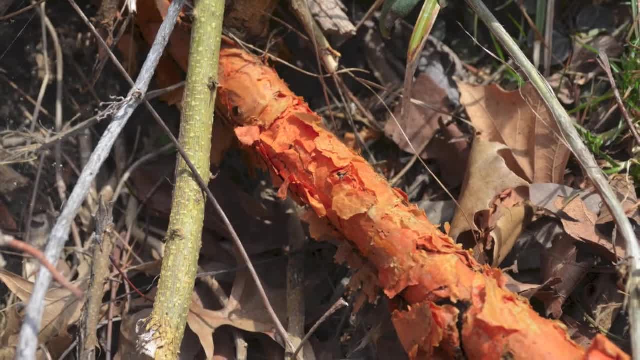 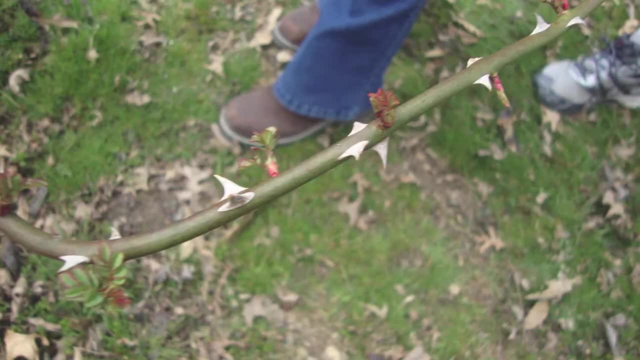 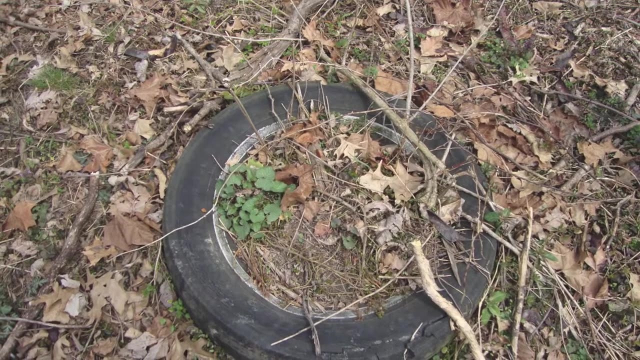 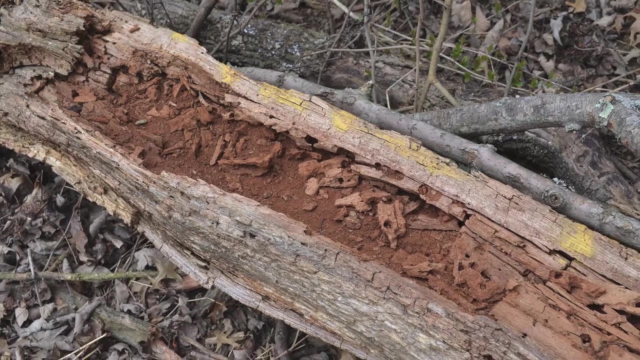 We send the seeds out in the breeze. We're coming down, Coming down to earth, Like babies at birth. Coming down to earth, We define our priorities. These are extraordinary qualities Down down, down to the ground. We're coming down to the ground. 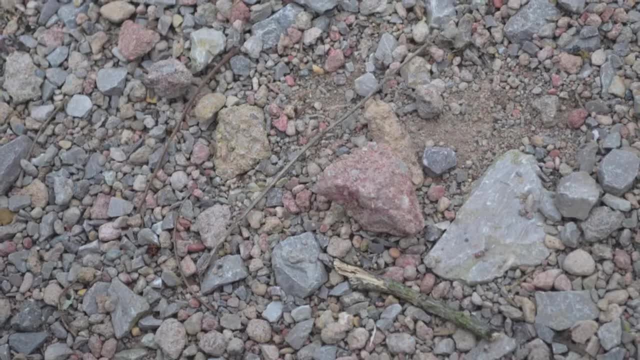 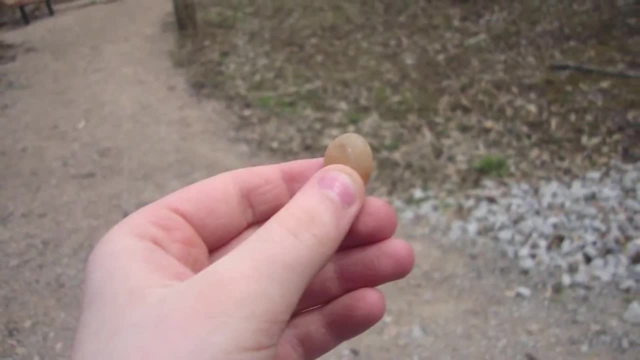 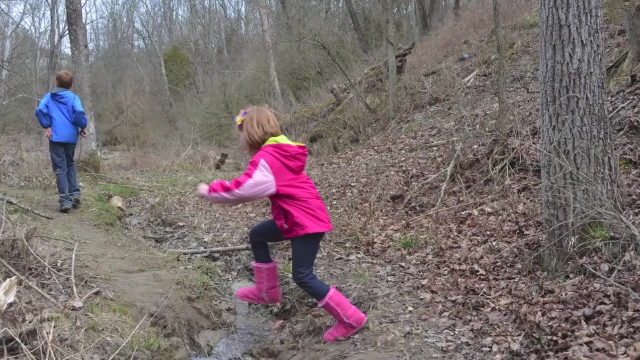 There's no better place to go. We've got snow upon the mountains, We've got rivers down below. We're coming down to the ground. Sometimes you may even find that the kids just want to put the camera down and do a little exploring all on their own. 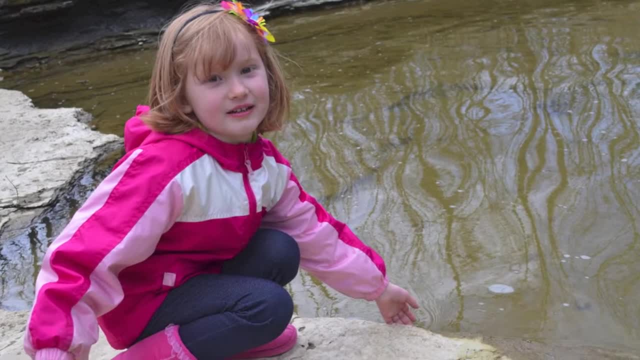 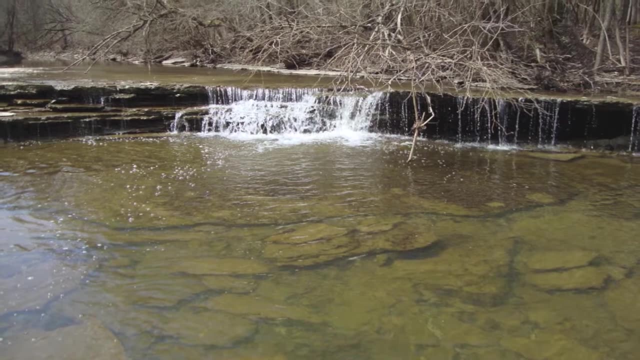 Which is perfectly natural, wonderful and exactly what we want to see happen- Coming down to the ground. There's no better place to go. We don't have to take away technology completely to address the disconnect issues that Richard Louv worries so much about. 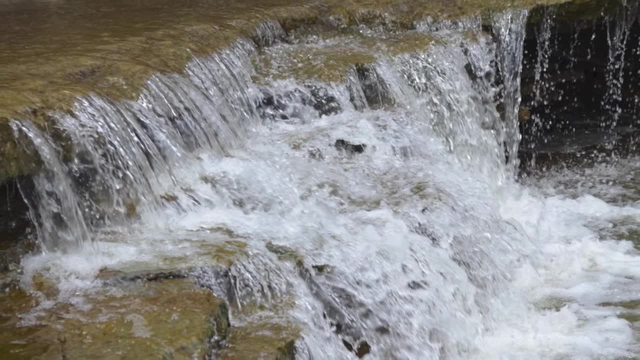 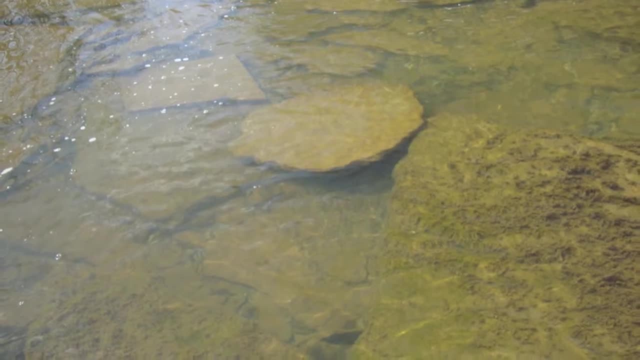 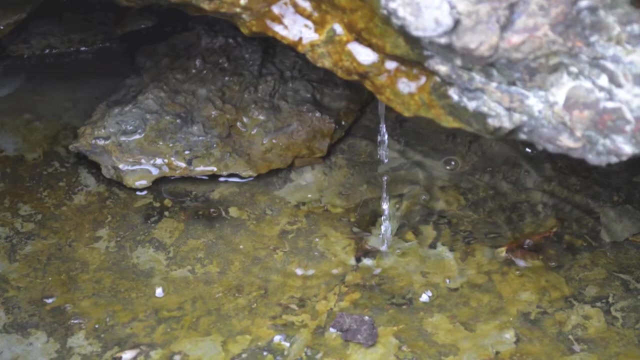 Coming down to the ground. We're coming down to the ground. There are few opportunities today for our children to do what they love to do, as opposed to doing what's required of them. If providing them with a digital camera and releasing them out into nature gives them an opportunity to self-direct their own lives and reconnect to nature at the same time, then our goal has been met. 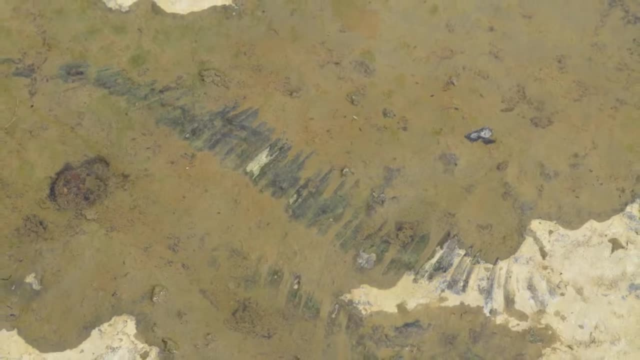 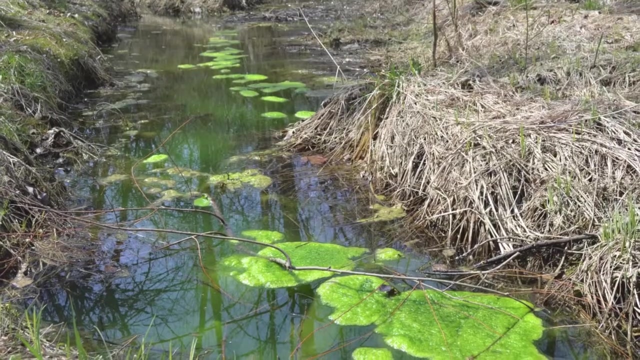 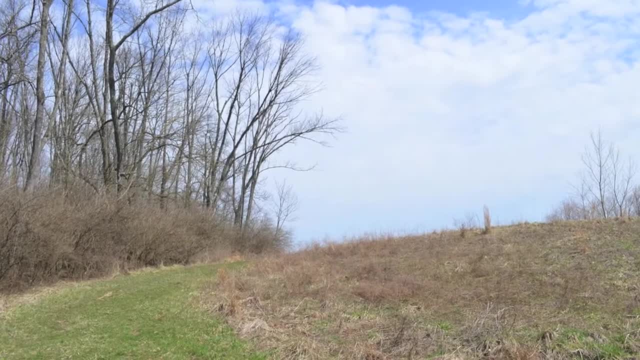 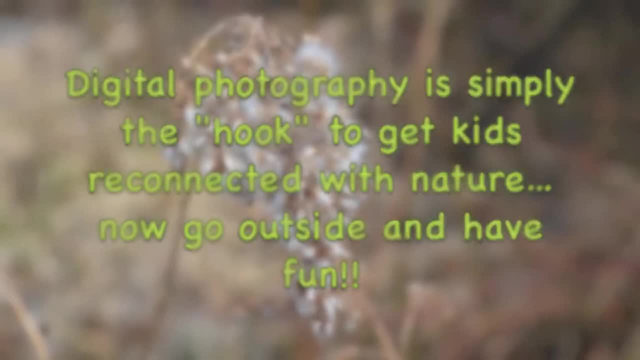 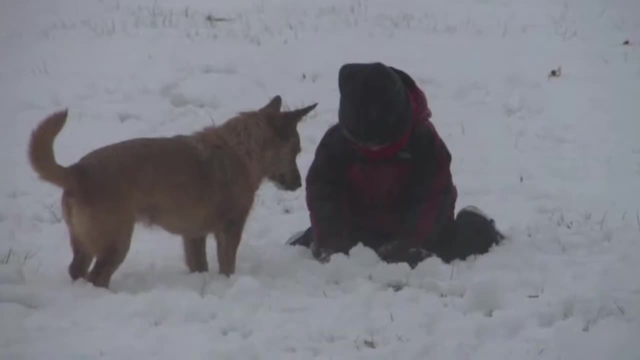 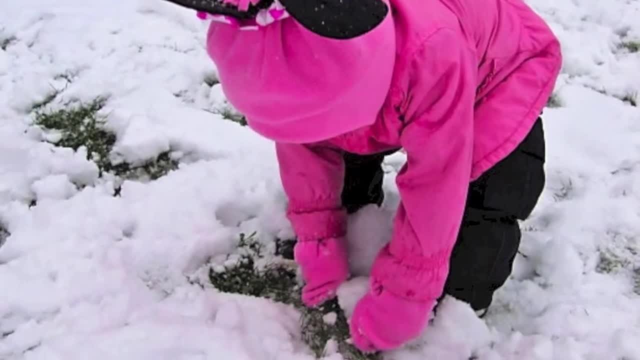 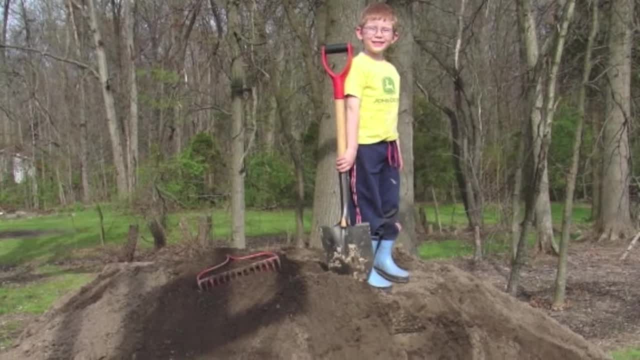 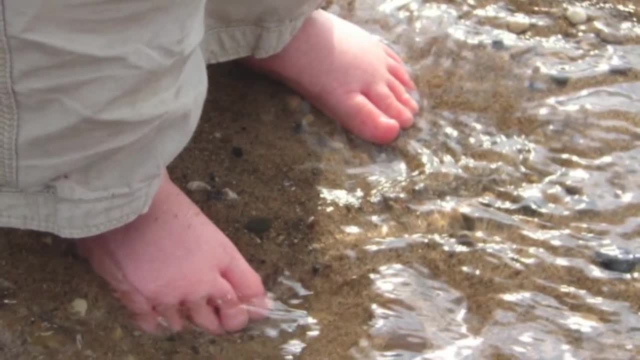 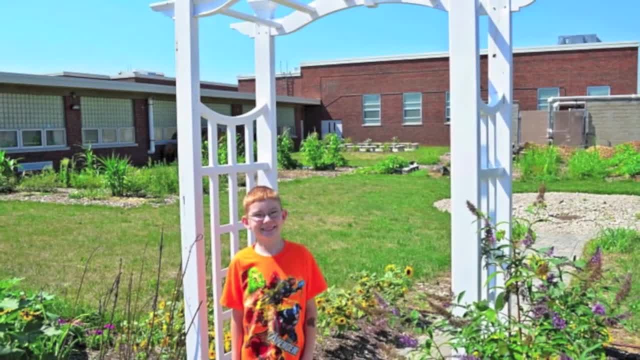